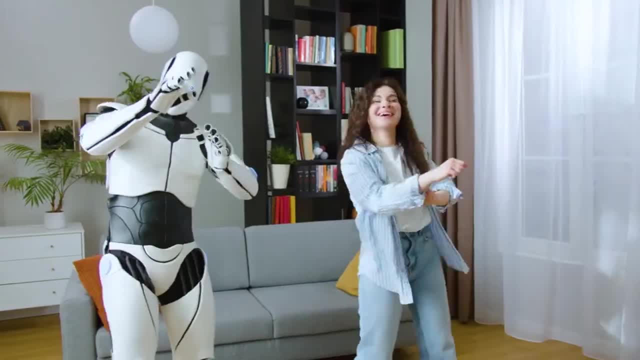 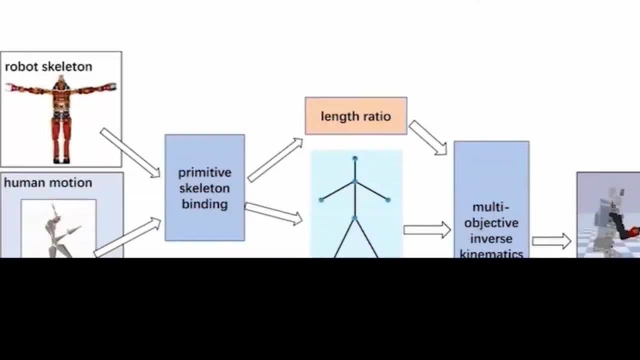 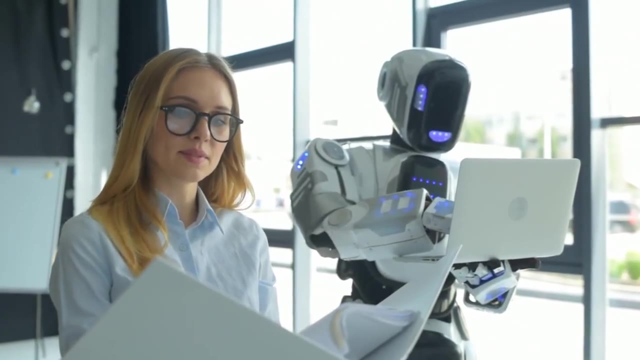 Human motion: a symphony of complexity. The elegance of human motion is a complex dance. It involves a perfect harmony of muscle activations, joint movements and intricate balance control. Human locomotion is a unique orchestration, finely tuned over millions of years of evolution, enabling us to navigate our physical world effortlessly. The Herculean task of 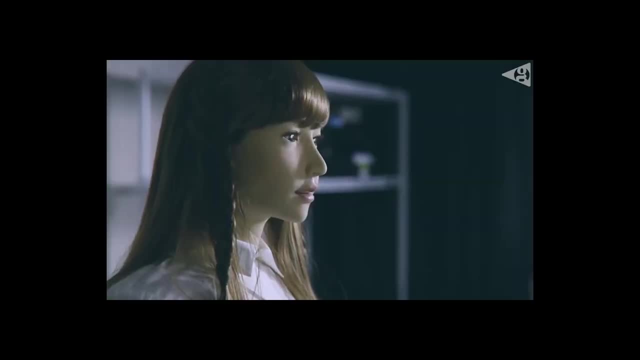 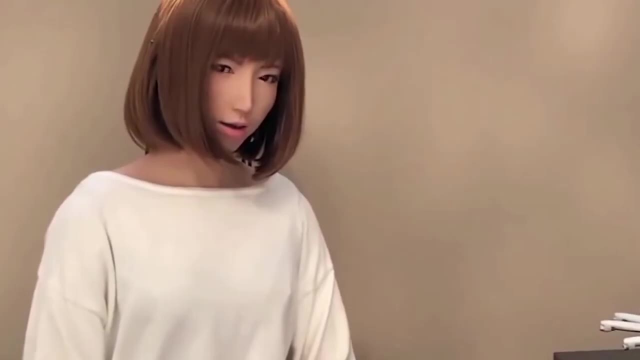 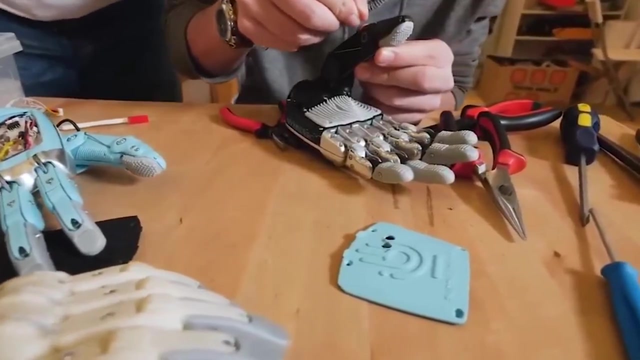 transferring human motion to robots. However, transferring this intricate symphony of locomotion and adaptive gait transitions to humanoid robots has always been a formidable task. The control complexity, coupled with the nonce motion design required, makes it a challenge that has stymied researchers for years. 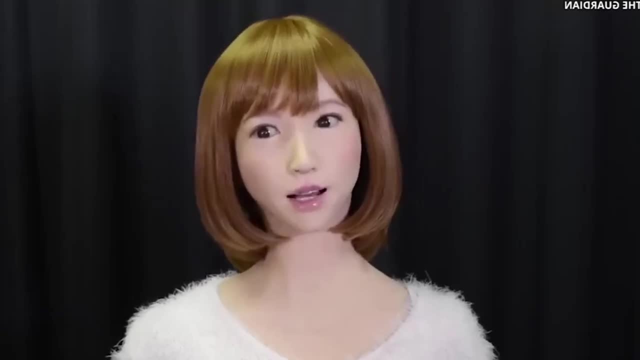 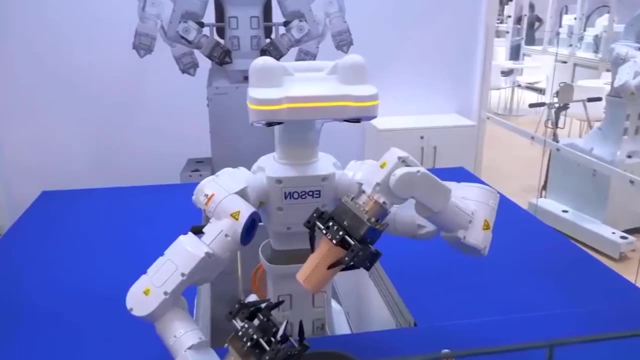 The Wasserstein Adversarial Imitation Learning System. In our exploration of this incredible system, we uncover how Wasserstein Adversarial Imitation Learning bridges the gap between human and robot. We'll explore the complexity of human motion and robotic movement. The system is a game-changer in the field of robotics, paving the way for 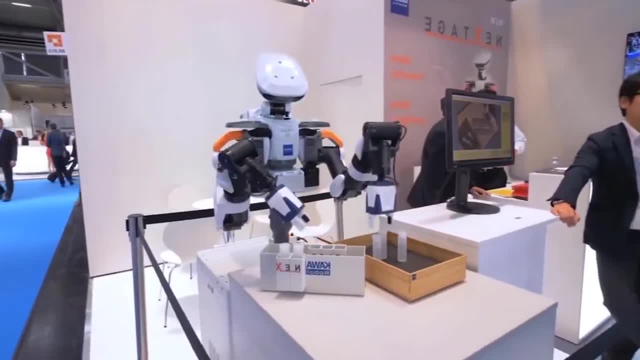 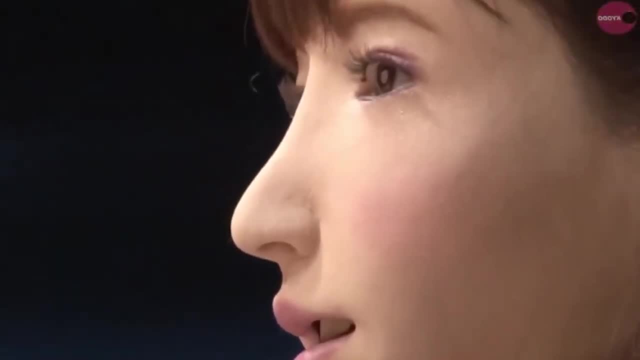 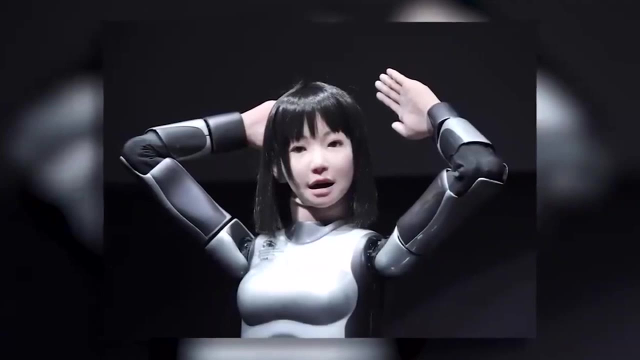 robots that move with unmatched fluidity and precision, closely mirroring human actions. The Significance of Human Mimicry in Robotics: To understand the full scope of this innovation, we delve into the significance of achieving human mimicry in the world of robotics. Beyond the technical aspects, we explore how this development 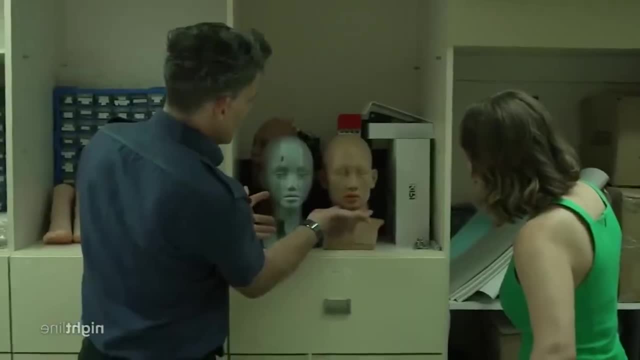 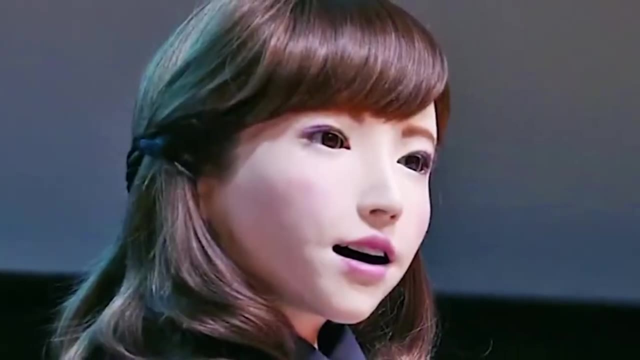 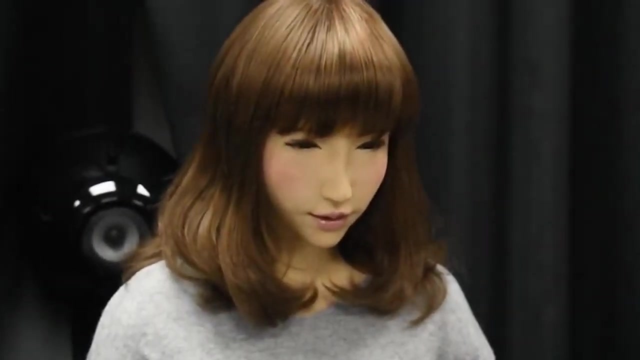 has the potential to revolutionize industries From healthcare to manufacturing, Bridging the Divide between Humans and Robots. The human form and that of humanoid robots have inherent differences. In this video, we unveil the unified primitive skeleton motion retargeting approach By incorporating the Wasserstein one distance and a pioneering soft boundary constraint. 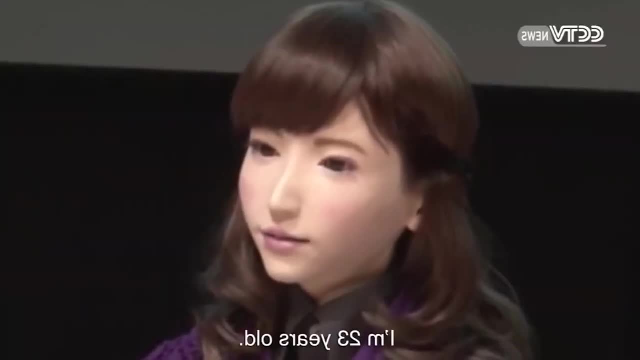 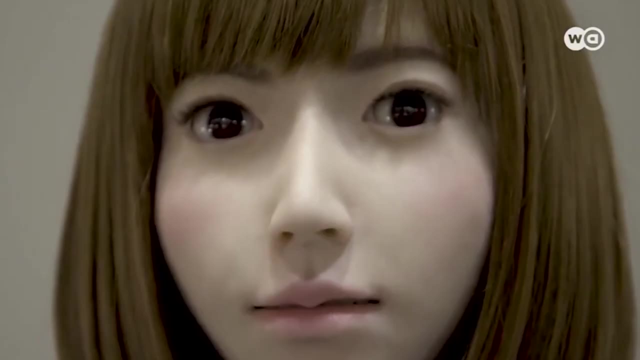 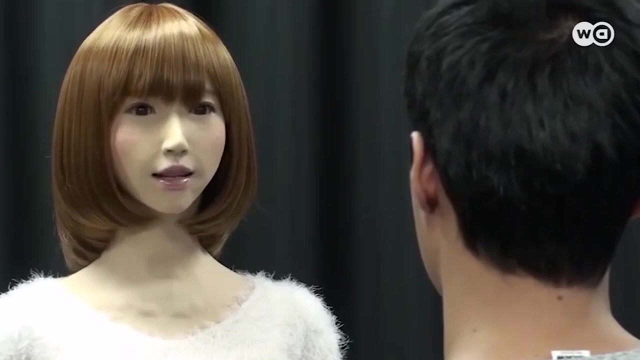 the researchers have managed to stabilize the training process and prevent model collapse. The result: A groundbreaking control policy that encompasses a spectrum of locomotion patterns From standing to dynamic running. Wasserstein One Distance- a key to success: The use of the Wasserstein One Distance integrated with a pioneering soft boundary. 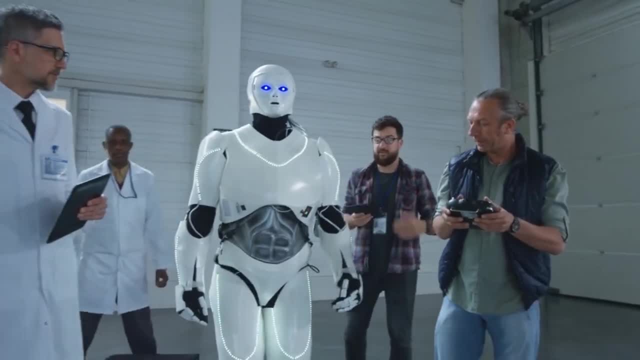 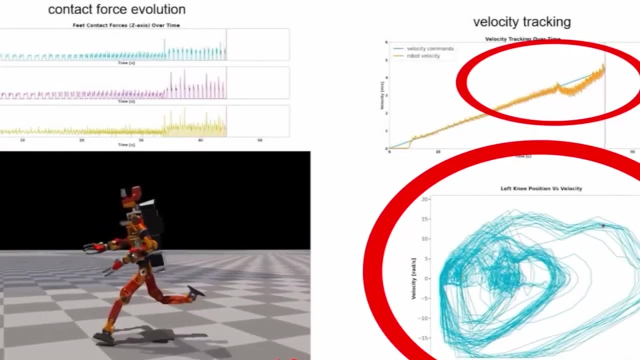 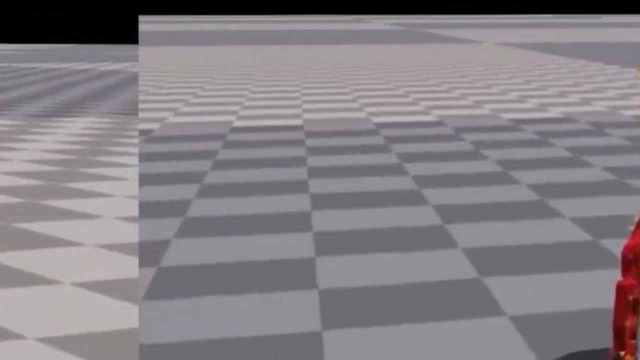 constraint was a game-changer. It allowed researchers to bridge the gap between the morphological differences of humans and humanoid robots. This breakthrough not only stabilized the training process, but also prevented model collapse. A spectrum of locomotion patterns. The forthcoming control policy is nothing short of revolutionary. 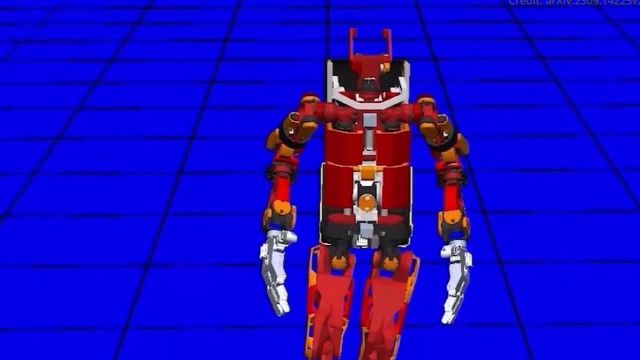 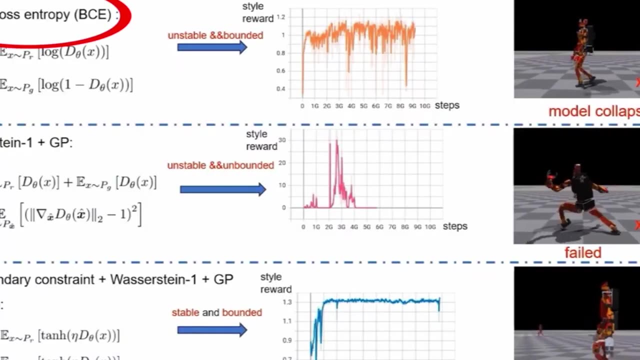 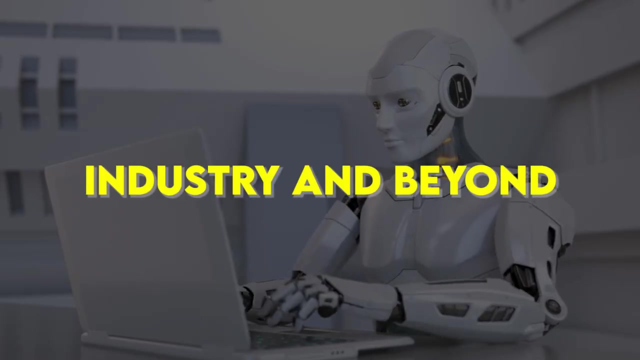 revolutionary. It includes a diverse spectrum of locomotion patterns, ranging from standing and push recovery to squat walking, human-like straight-leg walking and dynamic running. This versatility is a significant leap forward in the world of robotic locomotion, the impact on industry and beyond. Beyond the world of research, this achievement has far-reaching 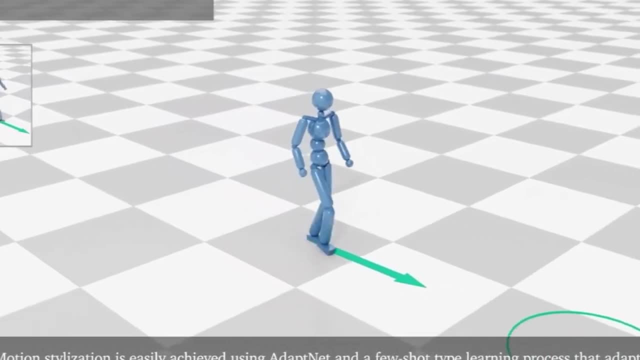 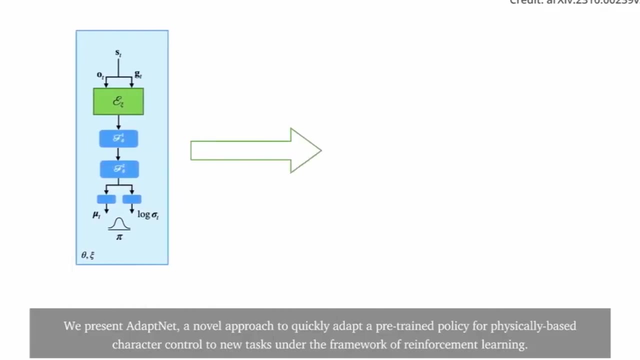 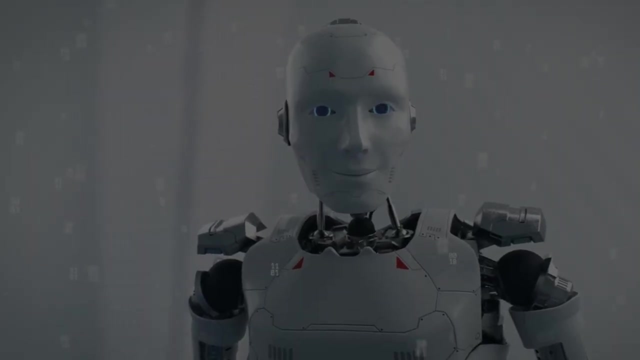 implications for various industries. We explore how this technology can enhance manufacturing, healthcare and even space exploration. Robots that can mimic human movements offer a level of dexterity and adaptability previously unseen. The Advent of AdaptNet. We introduce you to AdaptNet, a game-changing character control technique. This innovative 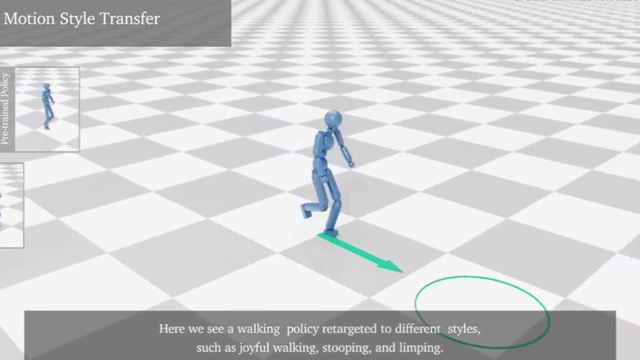 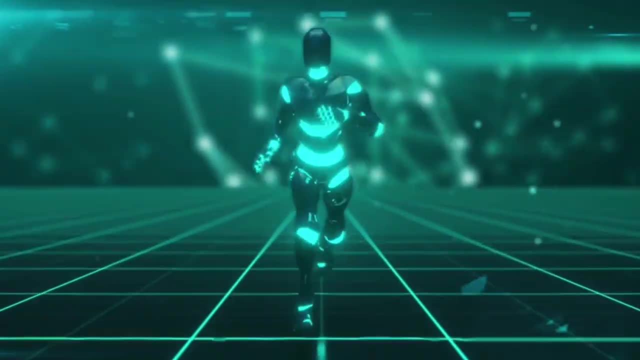 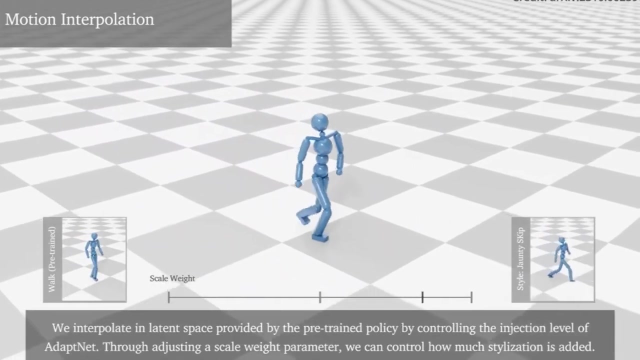 approach allows for quick policy adaptation, bringing about a seamless and efficient mechanism for skilled motion behaviors across various settings and tasks, From motion stylization to morphological and environmental adaptation. AdaptNet showcases its versatile capabilities. It can even achieve motion stylization in under 30 minutes, opening up a world of possibilities for creating diverse 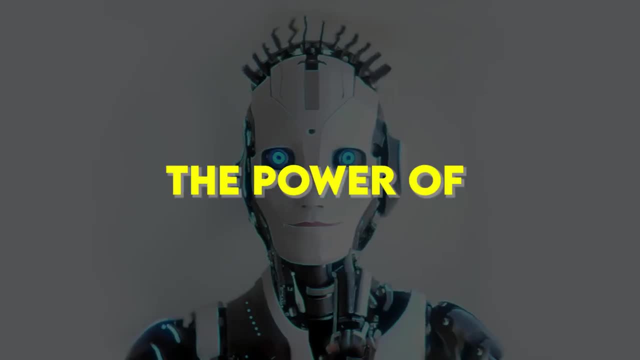 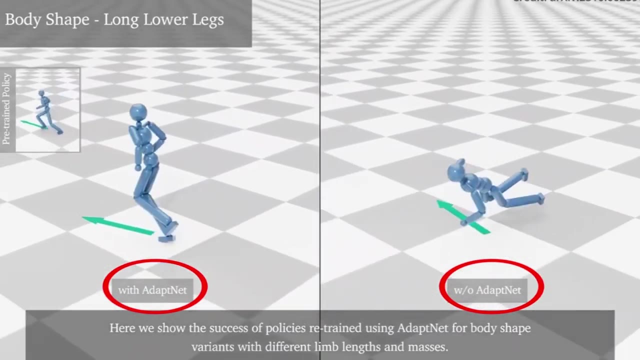 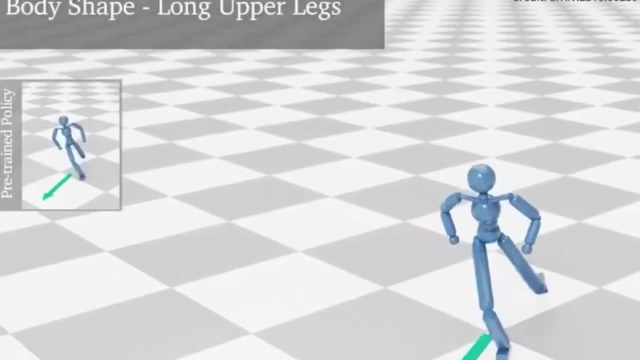 AI characters in virtual environments. The power of quick policy adaptation. AdaptNet's ability to adapt policies rapidly opens up new horizons in AI robotics. It allows robots to not only learn but also adapt on the fly, making them more versatile and efficient in real-world scenarios. 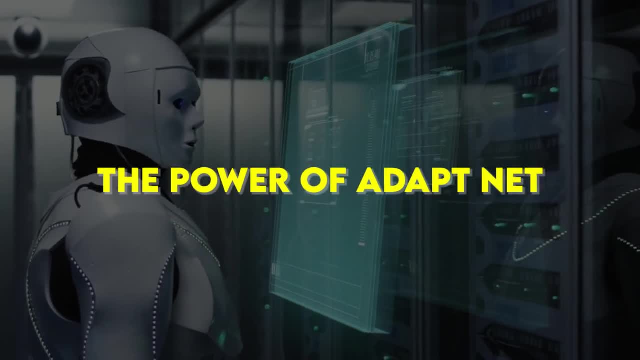 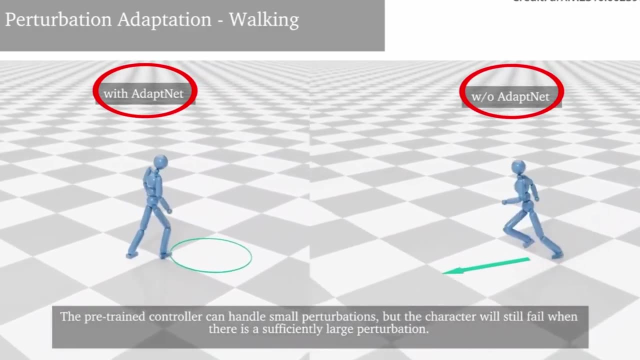 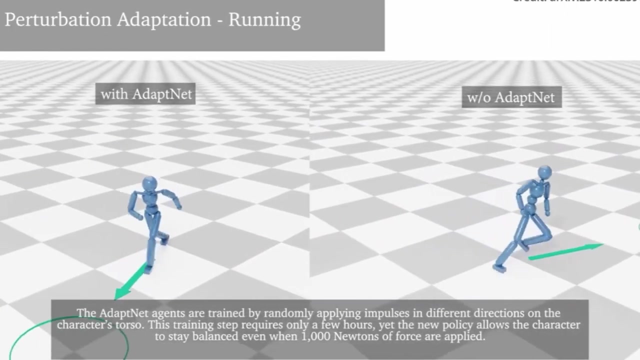 Customization and Robustness- The power of AdaptNet. AdaptNet doesn't stop at stylization. We explore how it smoothly interpolates between pre-trained policies and styled policies, offering a nuanced and customizable approach to motion generation and control. We'll also discover how AdaptNet efficiently adapts to 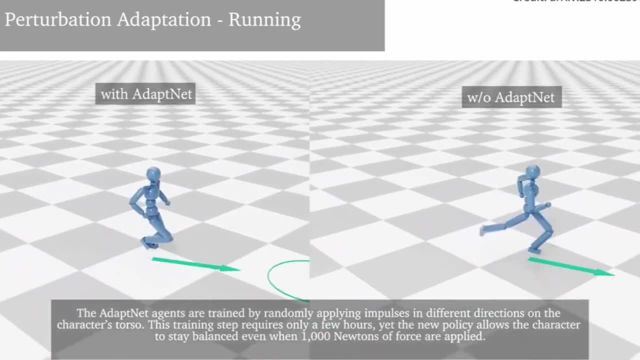 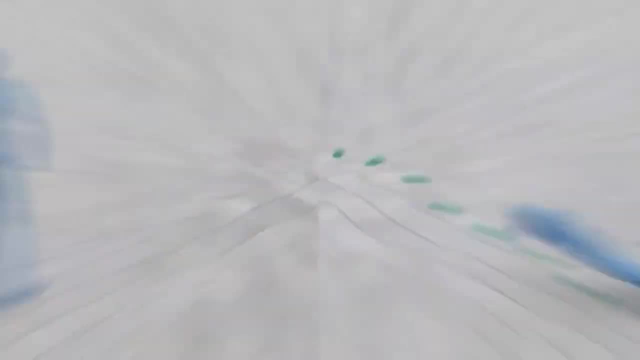 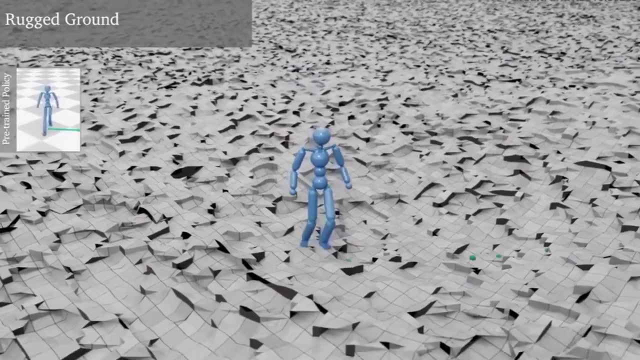 different character morphologies and dynamics. Its deep neural network ensures characters maintain balance and control even when faced with morphological changes. Customization for a World of Diversity: AdaptNet's ability to interpolate between different policies while adapting to diverse character morphologies and dynamics, showcases its potential to operate in an increasingly 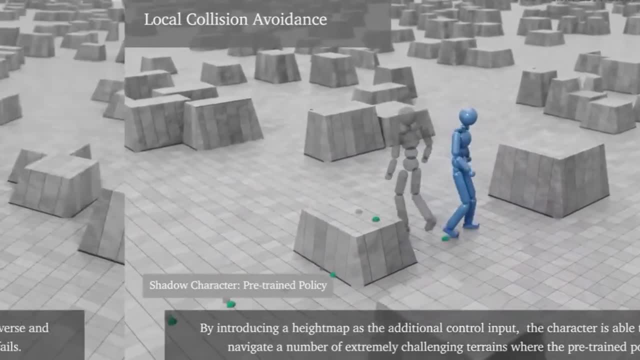 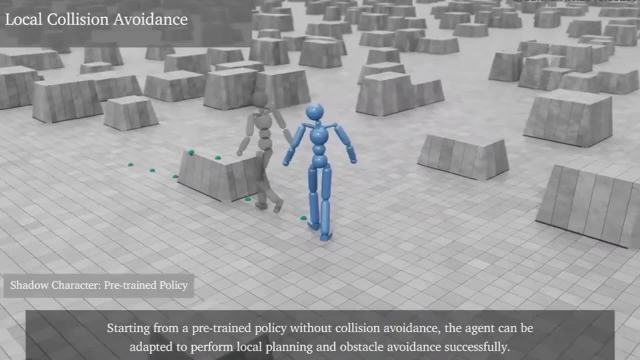 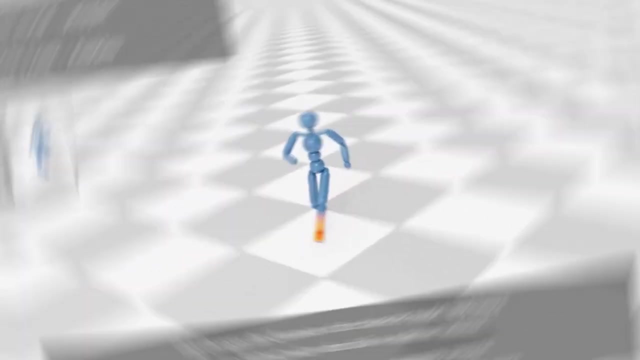 diverse world, From different body shapes to varying masses, this technology can adapt and excel, Adapting to the Unpredictable Navigating, Complex Environments. AdaptNet enhances the robustness of walking and running controllers With randomized impulsive impulses applied to the character's torso. these policies maintain balance, even. 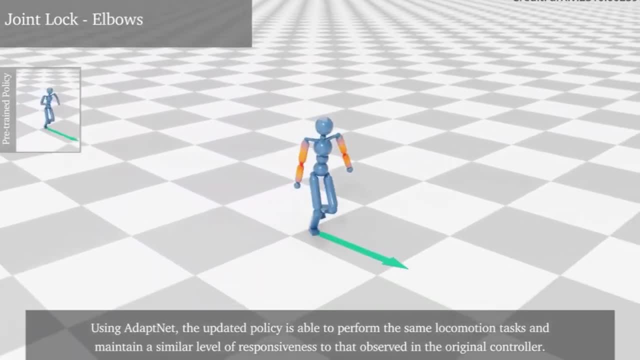 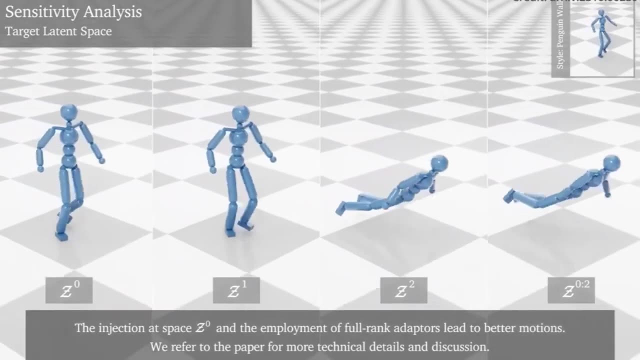 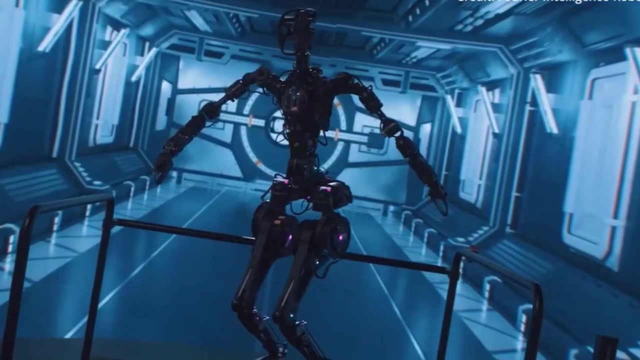 under substantial perturbations. Additionally, AdaptNet fine-tunes control policies to accommodate environmental changes, even in challenging terrains. The adaptability to environmental variables is truly remarkable. Robustness in the face of challenges. The ability of AdaptNet to navigate unpredictable challenges and maintain balance, whether through 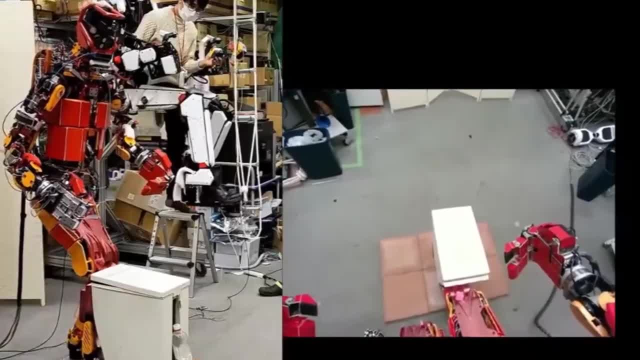 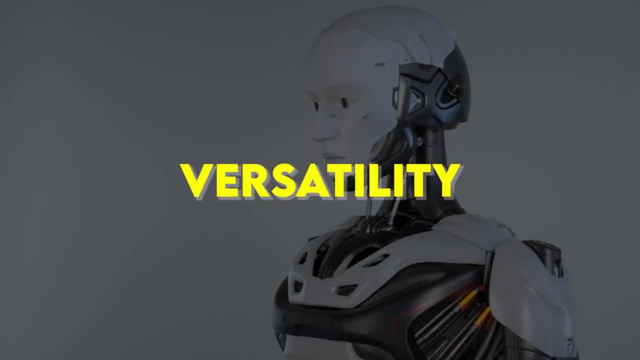 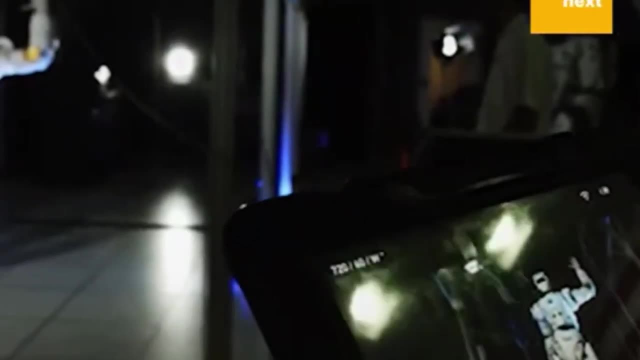 randomized impulses or changes in environmental factors is a testament to its resilience. This adaptability positions robots for success in real-world scenarios. Versatility in real-world scenarios: We'll explore how AdaptNet extends its capabilities to local planning and obstacle avoidance. Starting from a pre-trained policy without collision avoidance, the agent can adapt to. 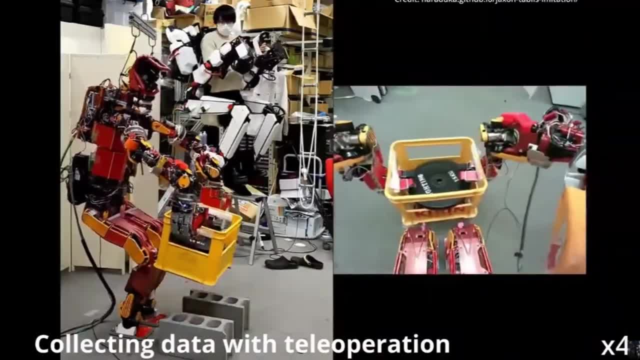 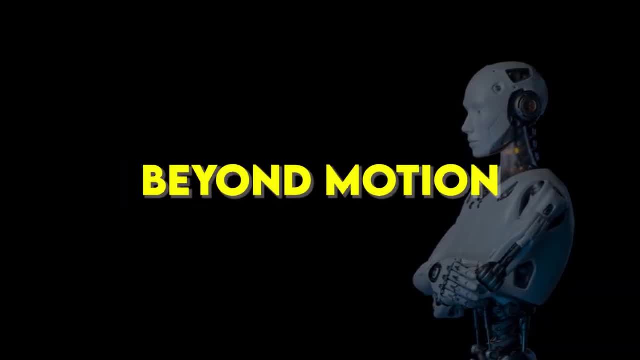 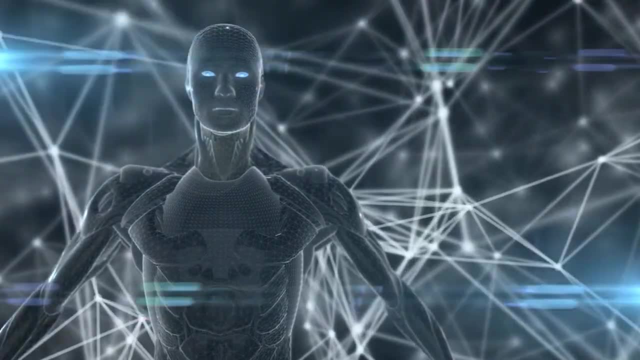 perform local planning and obstacle avoidance, demonstrating its versatility in real-world scenarios where obstacle navigation is crucial. Versatility beyond motion: Beyond motion control: this technology showcases its versatility in tasks such as local planning and obstacle avoidance. This adaptability positions robots for success in real-world. 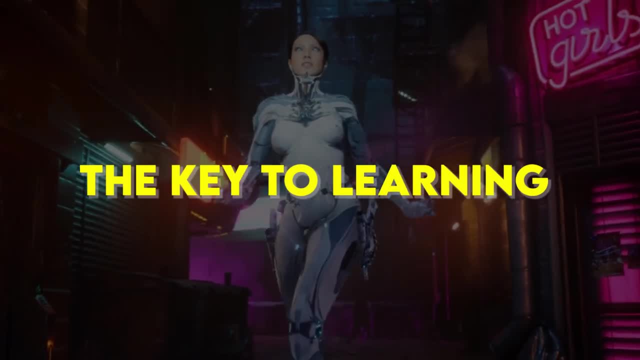 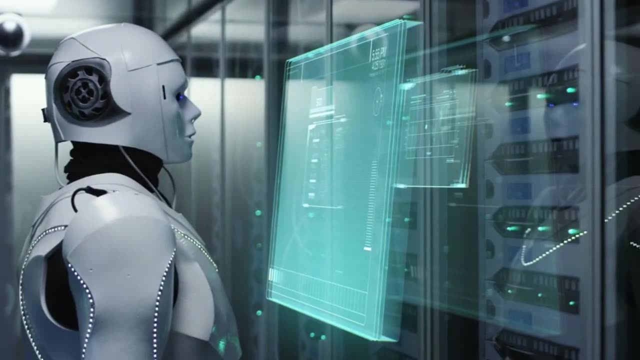 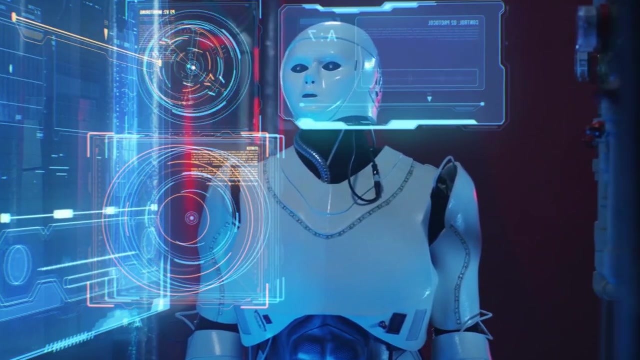 scenarios: Striking a balance: the key to learning stylized motions. Now we'll dive into the importance of striking a balance between avoiding overfitting and ensuring the learning of stylized motions. We'll discover how different regularization methods apply to the injected lead and play a vital role in ensuring the successful learning. 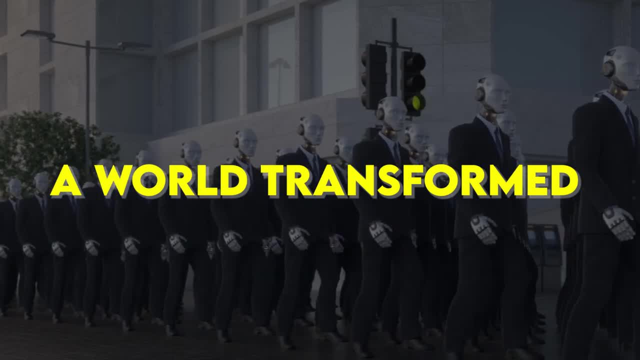 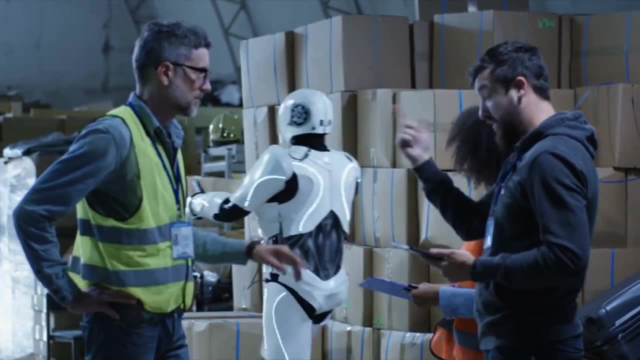 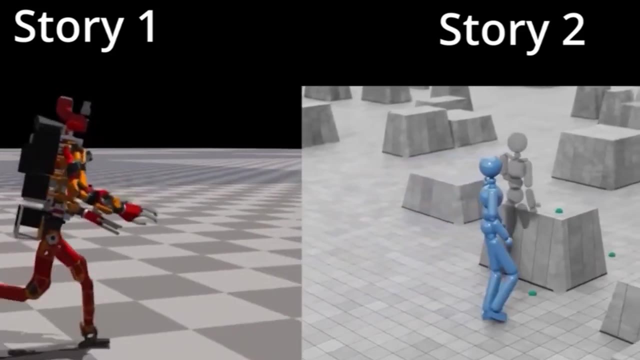 of stylized motions, A World Transformed – The Future of Robotics. As we wrap up our journey through these incredible techniques, we look at the implications of these advancements. The rapid progress of S13, adversarial imitation learning in AdaptNet paves the way for next-level teleoperation applications in robotics. We'll visualize: 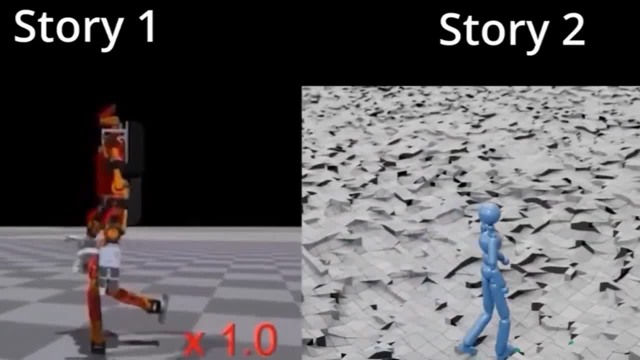